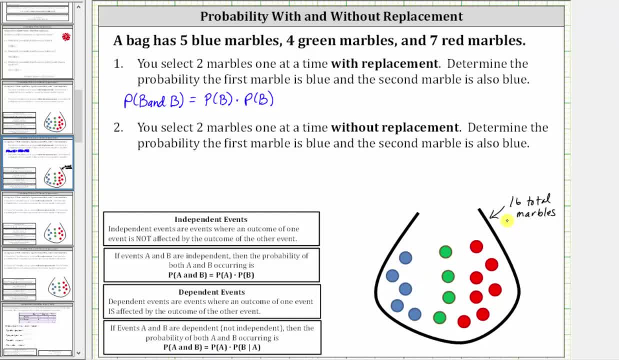 the probability of selecting of blue marble is 5 out of 16, or 5 16ths, which gives us 5 16ths times. again, the probability of something in blue marble is 5- 16ths. so we have 5 16ths times 5 16ths. 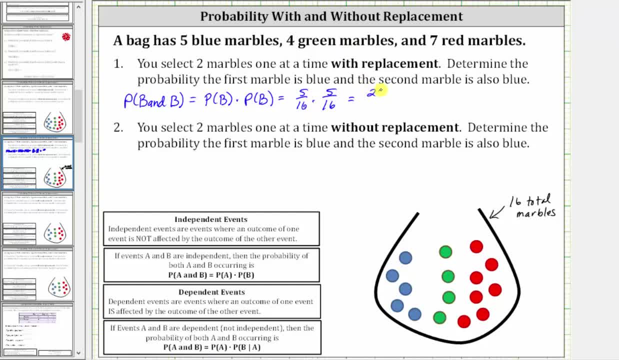 Nothing simplifies, and if we're multiplying, we have 25, 256, or 25 divided by 256.. Let's also express this as a decimal, in a percentage. In four decimal places, the fraction is approximately 0.0977,, which is 9.77%. 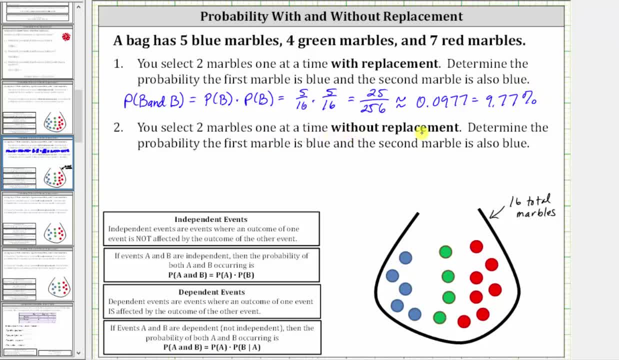 Now for the second example. you select two marbles, one at a time, without replacement, which means you select the first marble, do not replace it back into the bag and then select the second marble And we're asked to determine the probability. the first marble is blue and again the second. 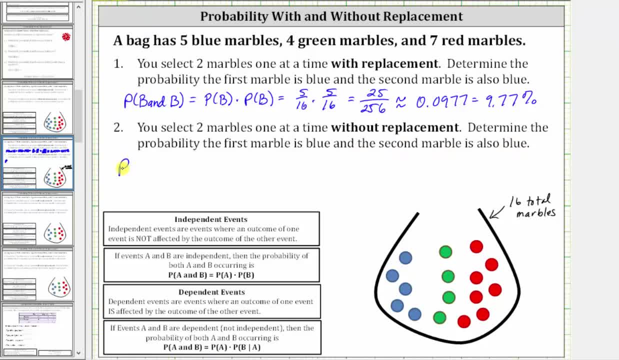 marble is also blue. So we want the probability of a blue marble And we want the probability of a blue marble, Another blue marble, but now without replacement. So, because the first marble is not replaced, back into the bag, the outcome of one event. 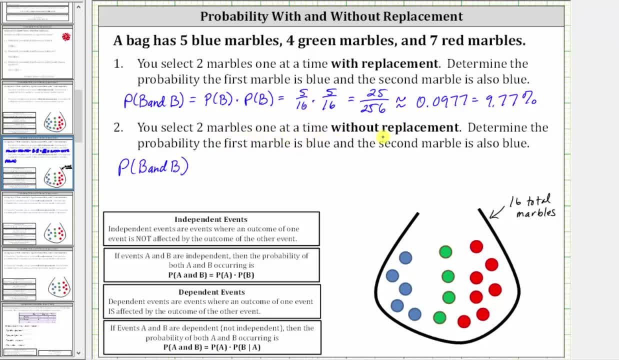 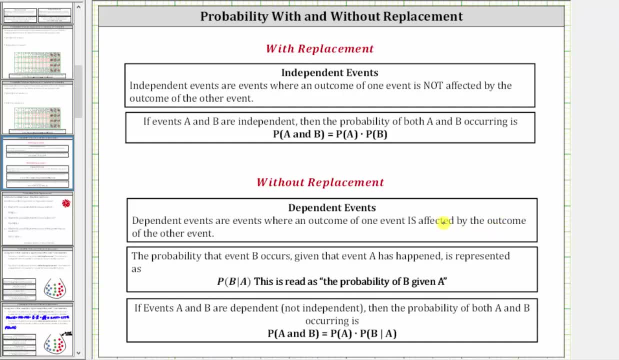 is affected by the outcome of the other and therefore now we have dependent events, Where dependent events are events where an outcome of one event is affected by the outcome of the other event, And the probability that event B occurs, given event A has happened, is represented using 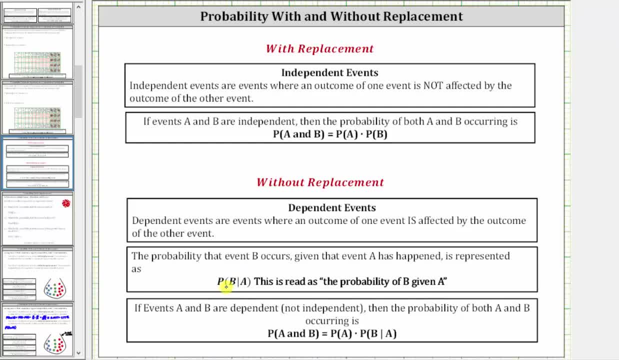 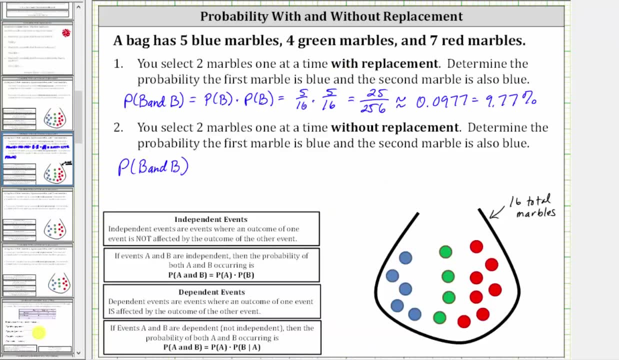 this notation here, which is read: If event A and B are dependent, the probability of both A and B occurring is equal to the probability of A times the probability of B given A has occurred. So, again for our example, because we have dependent events, the probability of B and 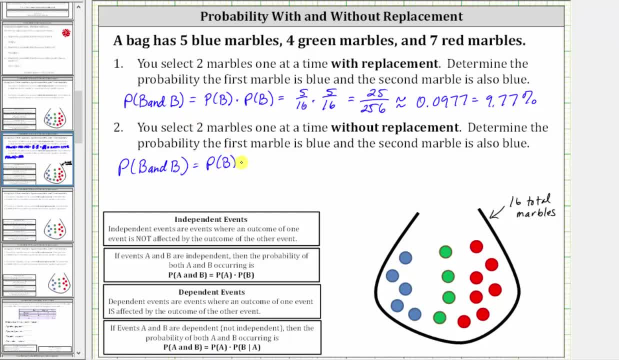 B is equal to the probability of B times the probability of B, given B has occurred. know from Part A. the probability of selecting a blue marble is 5- 16ths. But in this case a blue marble is selected and not replaced back into the bag before we. 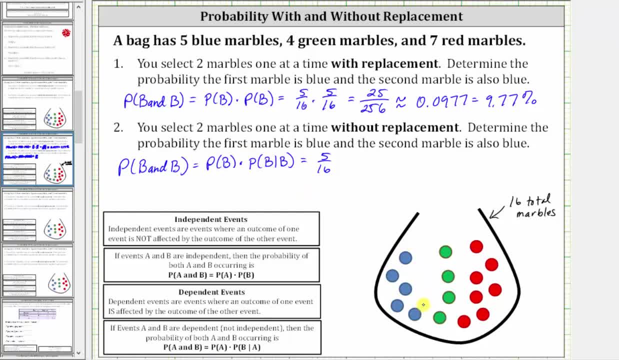 select the second marble. So let's just say this is the first blue marble selected, Because it's not replaced back into the bag now. we have a total of 15 marbles And now only four of the 15 marbles are blue And therefore the 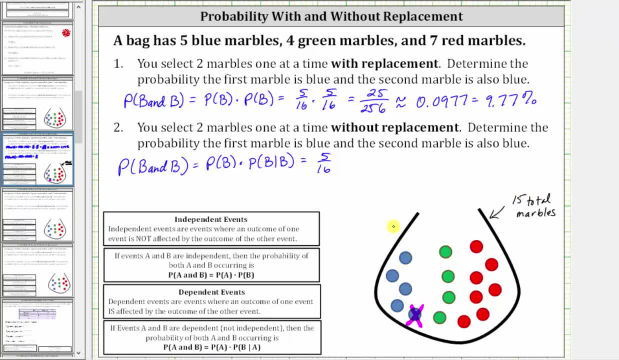 probability of selecting a blue marble- given a blue marble has already been selected and not replaced- is 4 out of 15, or 4 15ths. So notice how the number of favorable outcomes has decreased by 1 and the total number of marbles is also. 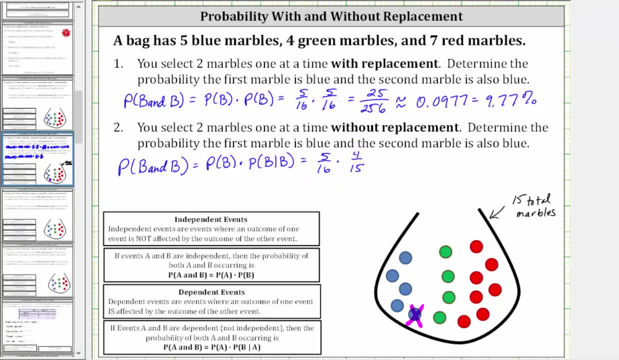 decreased by 1.. For multiplying, notice how we can simplify. There's a common factor of 4 between 4 and 16.. There's 1, 4 and 4 and 4, 4s and 16.. There's also a 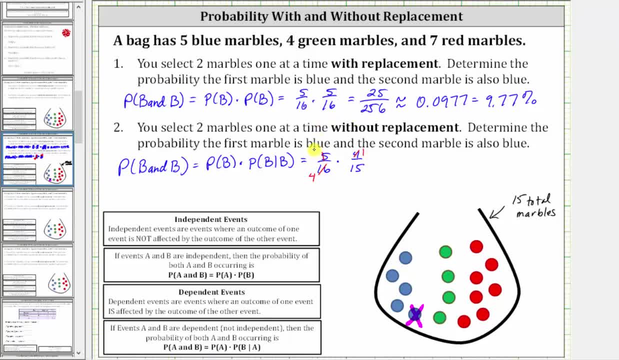 common factor of 5 between 5 and 15.. There's 1, 5 and 5 and 3, 5s and 15.. Multiplying the probability is 1- 12th. So the probability of selecting a blue marble and then another blue marble. 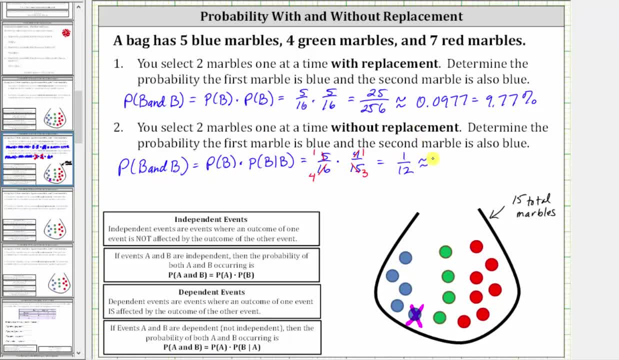 without replacement, is 1- 12th. Let's also show the decimal in percentage To 4 decimal places. 1- 12th is approximately 0.0833, which is 8.33%. I hope you found this helpful. 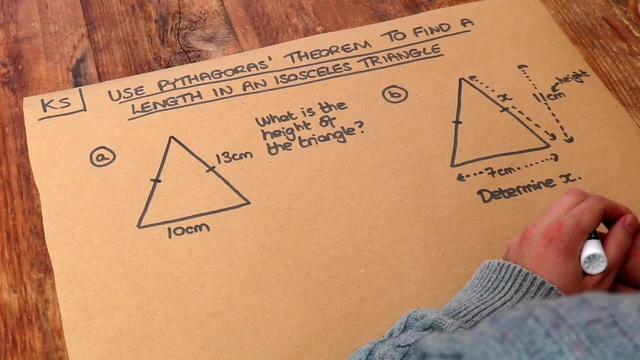 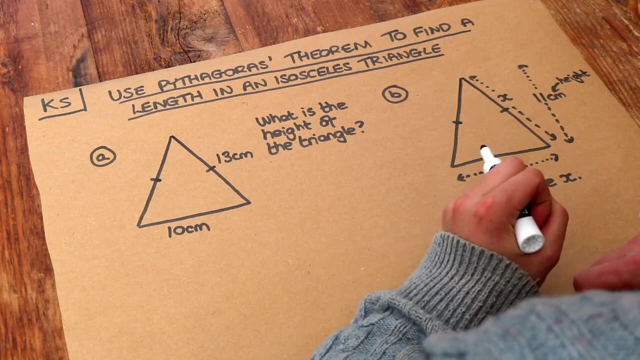 Hello and welcome to this Dr Frost-Maskey skill video on using Pythagoras Theorem to find a length in an isosceles triangle. Now remember, Pythagoras Theorem involves the right angle triangles. but these triangles here, they don't have a right angle, do they? 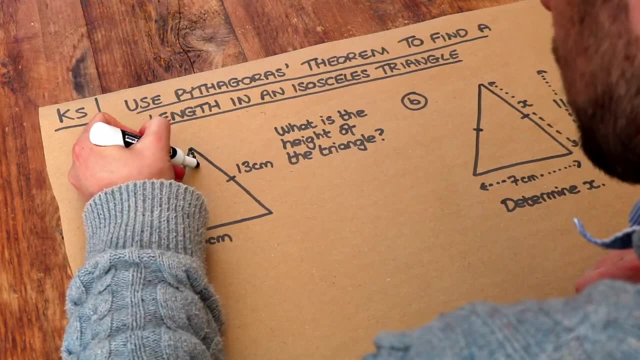 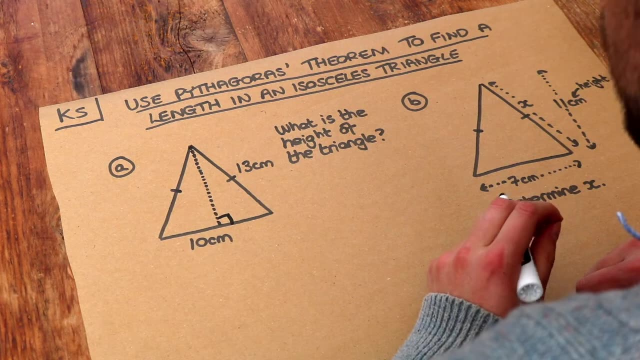 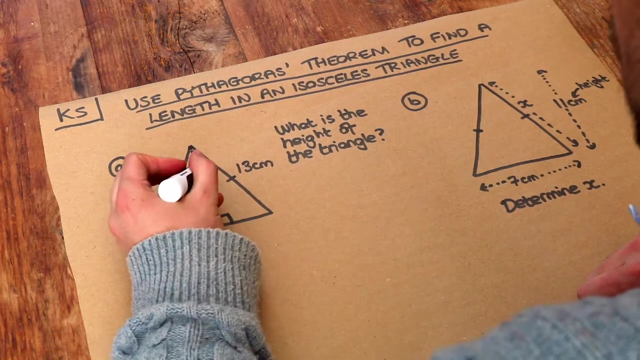 But if we were to split an isosceles triangle in two down its line of symmetry, can you see that we now have a right angle triangle? So we want to find the height of this particular triangle, this length here. Well, do we have two of the lengths of this particular triangle? Let's just say we use this half of it.